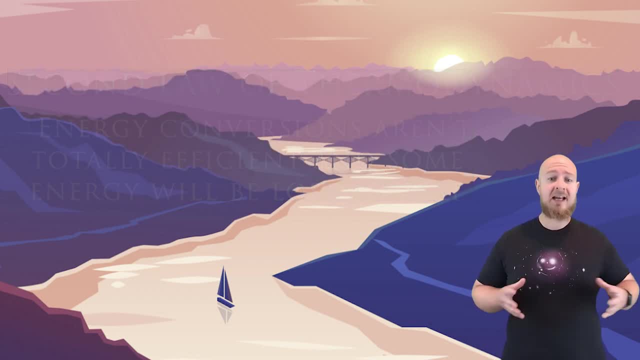 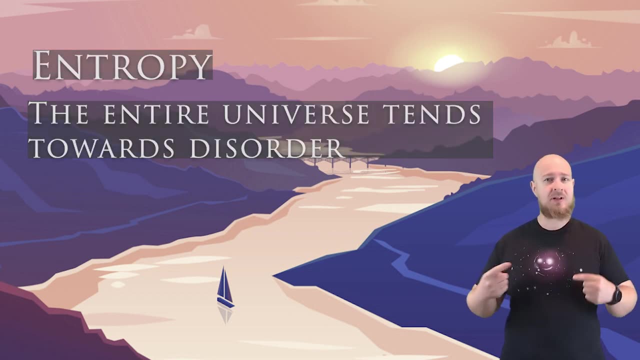 This is due to a property of the universe called entropy, where the entire universe tends towards a disordered state, and heat is a very disordered type of energy. Now, a deep understanding of entropy is not required for this class, but if you are interested in the description, 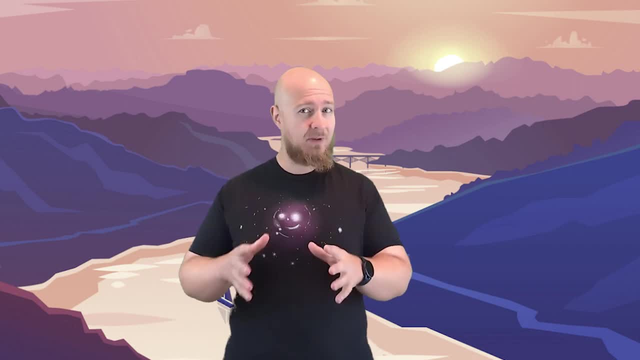 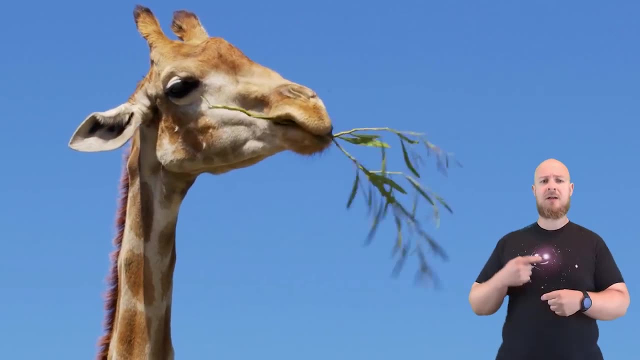 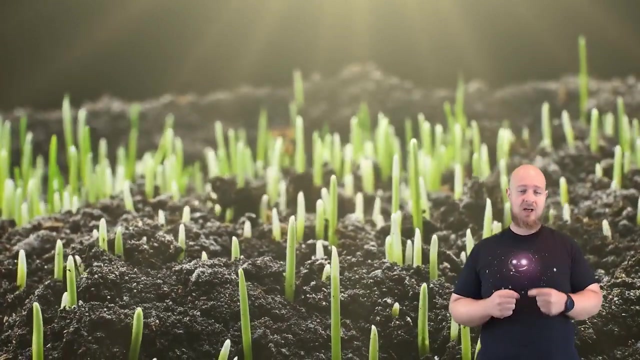 I linked a great video from TED-Ed that explains this concept very well. Energy, much like the elements we discussed during biogeochemical cycles, also cycles through the environment. Virtually all energy used in biological systems originates from the sun and is made available to living. 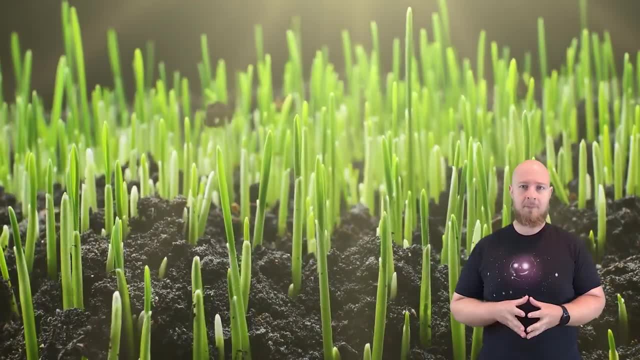 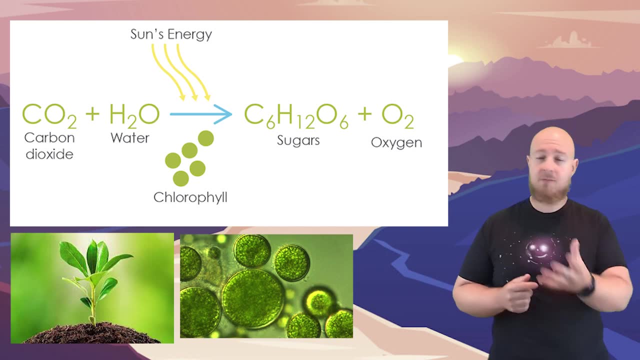 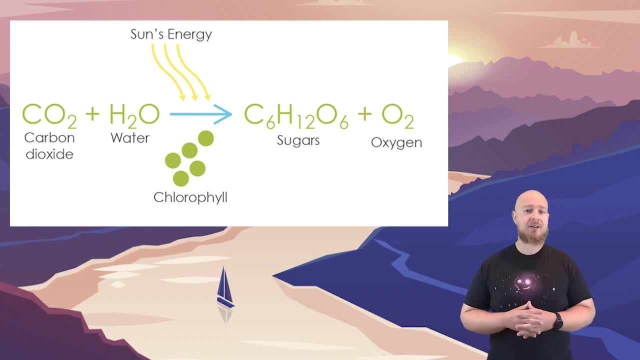 things through the process of photosynthesis. We've all seen this equation before right. Photosynthesis is the process that plants, algae and a few microbes use to make their own food. These organisms use the energy of the sun to react carbon dioxide with water to produce glucose and 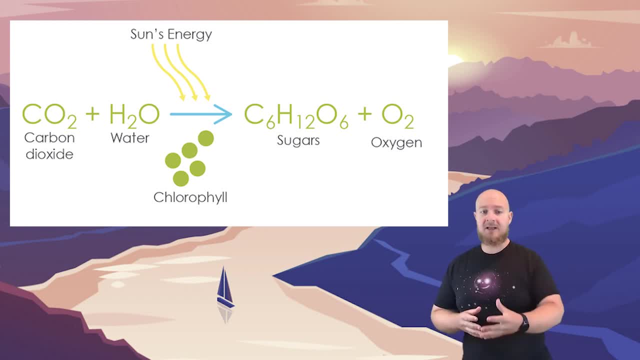 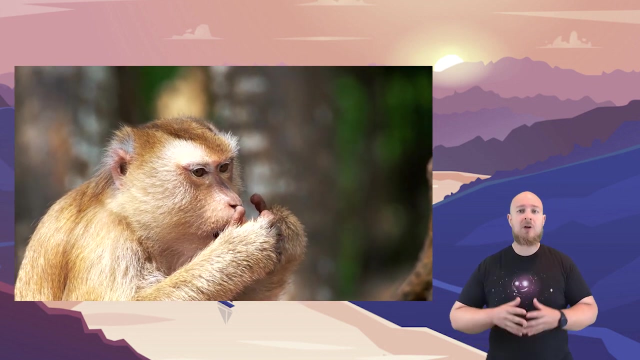 oxygen. The energy conversion that's happening here is this: The energy from sunlight is now being stored as the energy that holds together the chemical bonds of glucose. When plants then use that glucose to grow or when you eat them as food, you are converting that stored chemical energy and glucose to kinetic energy as you move around. 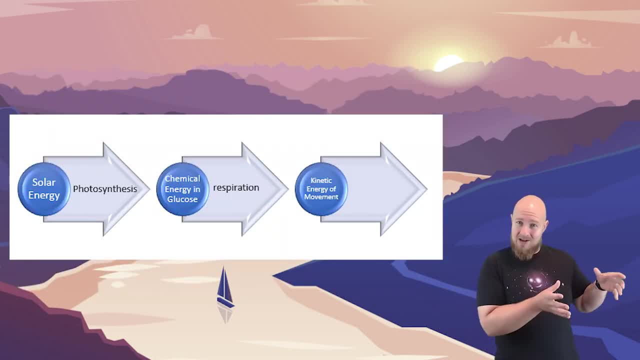 I made a fancy flow chart to show you what's happening here. right, Solar energy, energy from light, is now being stored in the chemical bonds of glucose. When you use that glucose for energy, you are converting that chemical energy to the kinetic energy of movement. 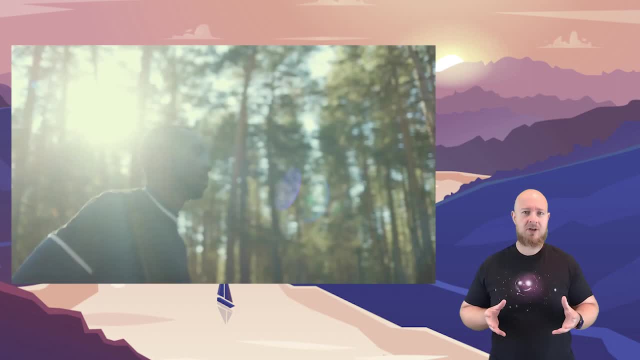 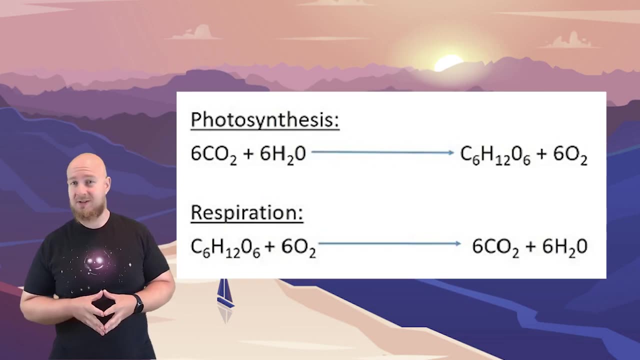 Using glucose to produce energy is called respiration, and I want to point something out about the photosynthesis and respiration. Let's take a look at these two equations. They are simply the inverse of each other. In photosynthesis, energy is being absorbed to 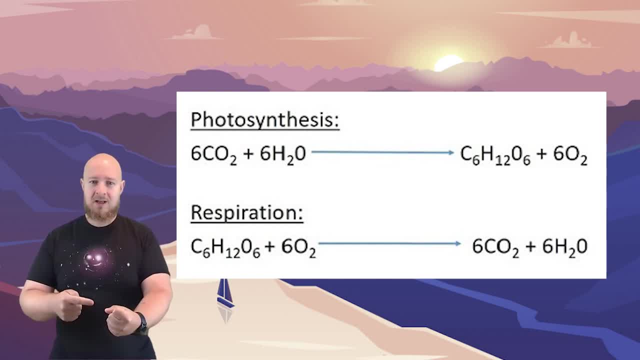 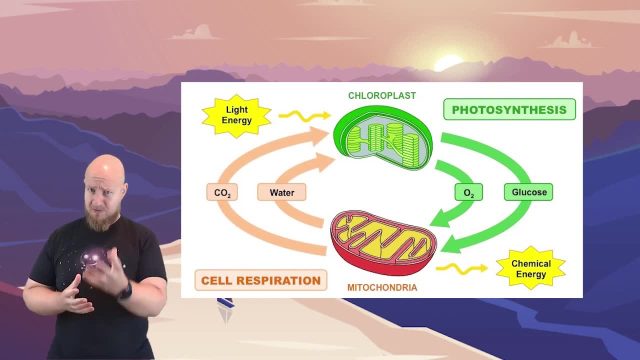 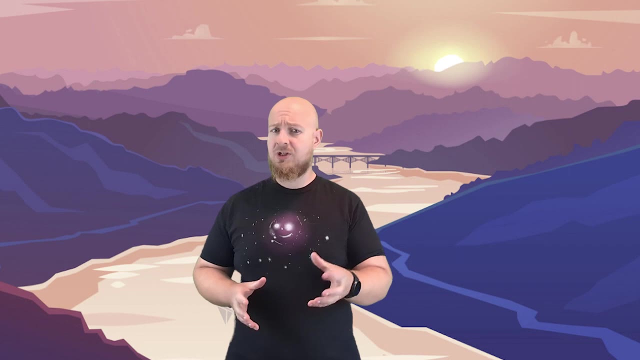 produce glucose and oxygen In respiration. that energy is released by the energy from the sun. When energy is released by the reaction of glucose and oxygen, to me this is remarkably profound. Energy is literally cycling in between these two processes. So let's take a look at how energy 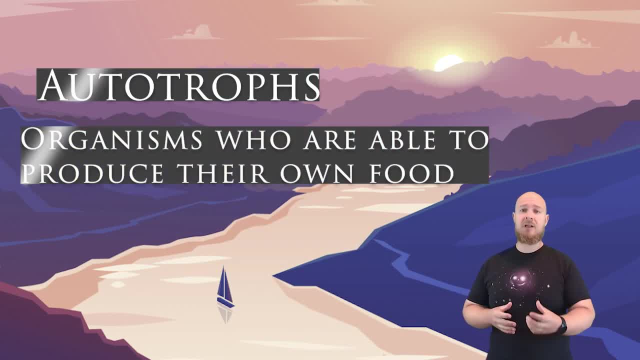 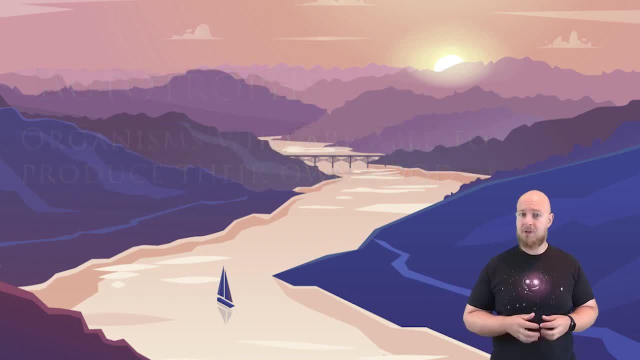 cycles through an entire ecosystem. All energy is made available to an ecosystem by producers. Producers are autotrophs or organisms who are able to produce their own food. Ecologists can measure the amount of energy being made available to an ecosystem's 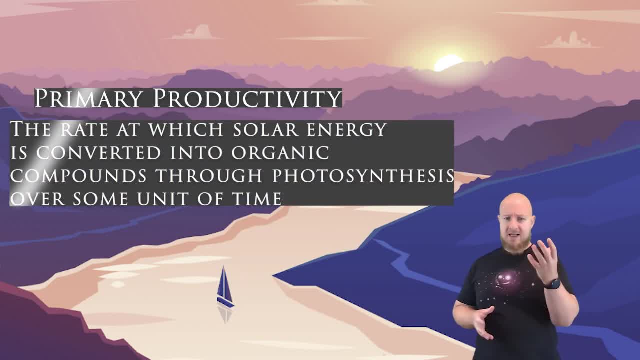 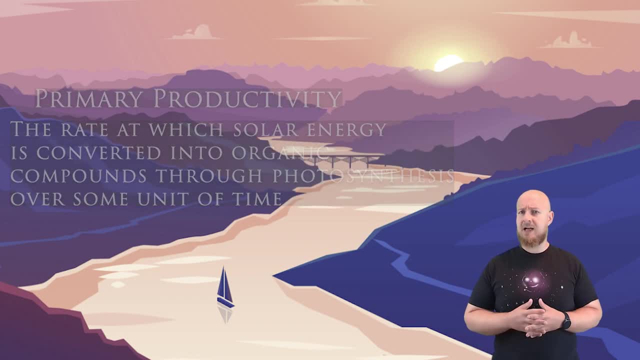 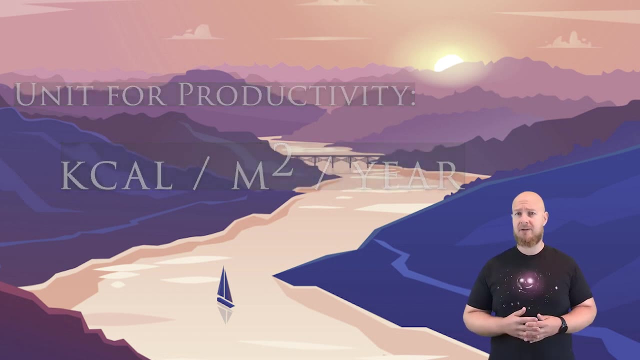 autotrophs. Primary productivity is the rate at which solar energy is converted into organic compounds via photosynthesis over some unit of time. Most commonly, this is represented by the amount of calories being produced every square meter every year. Gross primary productivity is the total rate of photosynthesis. 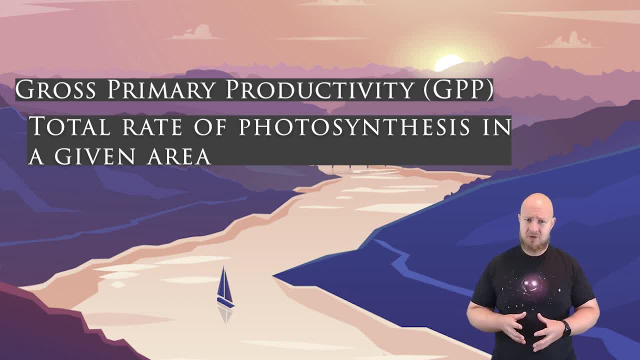 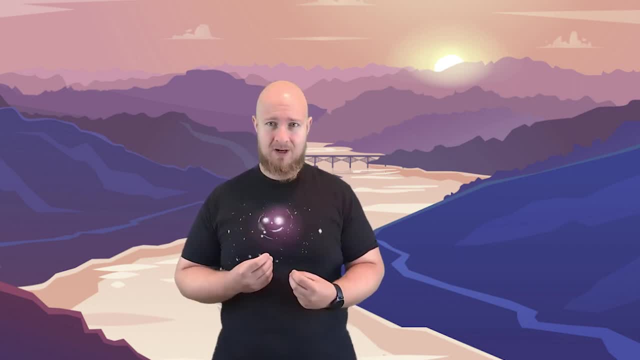 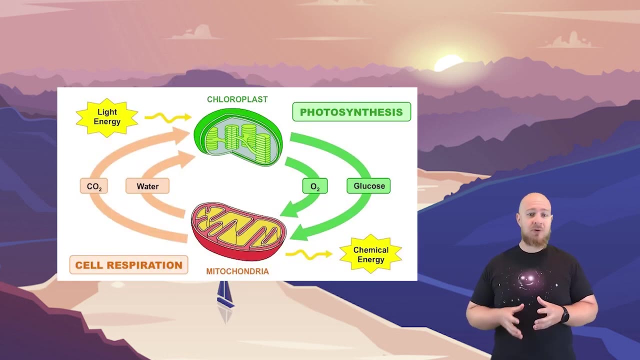 in a given area. However, not all of that energy is immediately available to the rest of the ecosystem. Plants do sure make glucose, but they also use it. Plants have mitochondria too, and undergo respiration, just like you and me. Plants use the glucose they make to power their 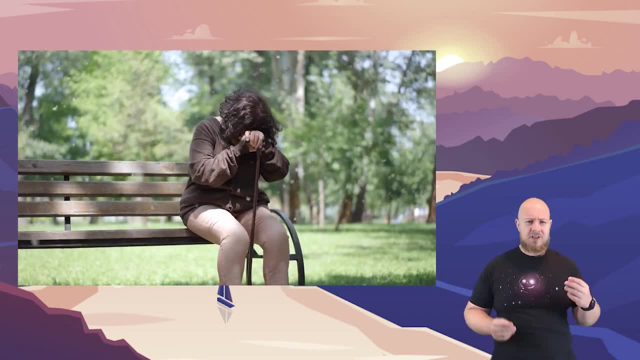 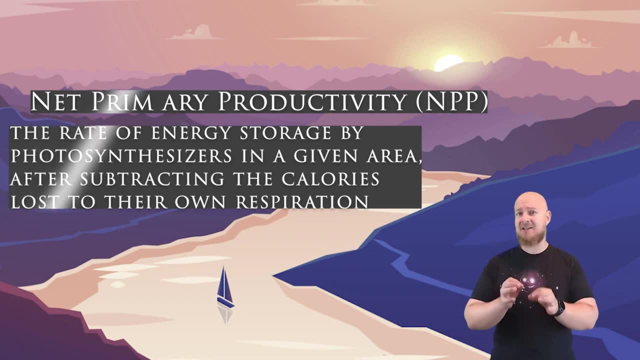 own plant life, things like growing and producing pollen, which causes my allergies. This is why the measure of productivity we look at in ecosystems is net primary productivity, The rate of energy storage by photosynthesizers in any given area, subtracting the energy lost to their own respiration, and this can be represented. by the formula: net primary productivity is equal to gross primary productivity minus the respiration rate. I do want to make it clear: plants don't produce glucose for you. Plants don't produce oxygen for you. The entirety of biological life on this planet is supported because plants and algae on the off chance. 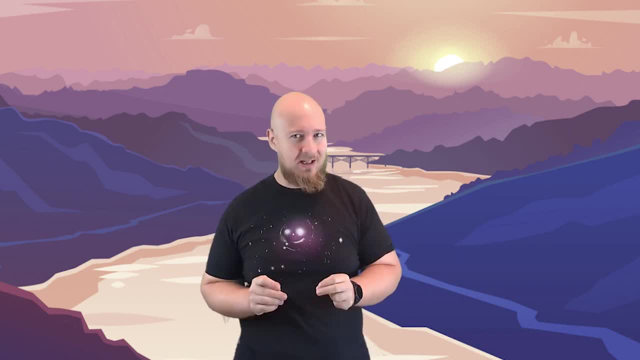 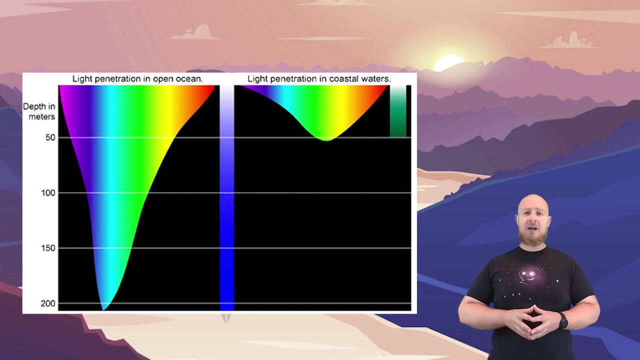 produce just barely more oxygen than they actually need for themselves. We are not that special. That's a good dark turn In aquatic ecosystems. the productivity does get a little bit trickier. Many photosynthesizers rely almost completely on two colors of light to do photosynthesis: red and blue. 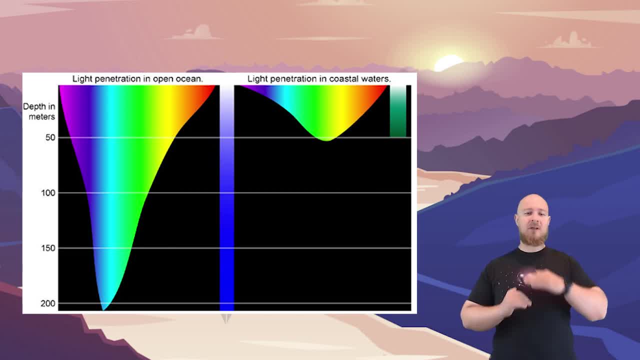 Red wavelengths of light are absorbed by the top 1 meter of water, and blue wavelengths of light can only penetrate about 100 meters in even the clearest of water conditions. this pretty much limits the area where photosynthesis can effectively make energy to the top few meters of the water. 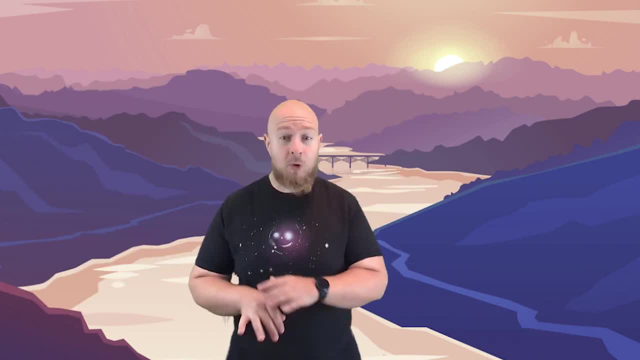 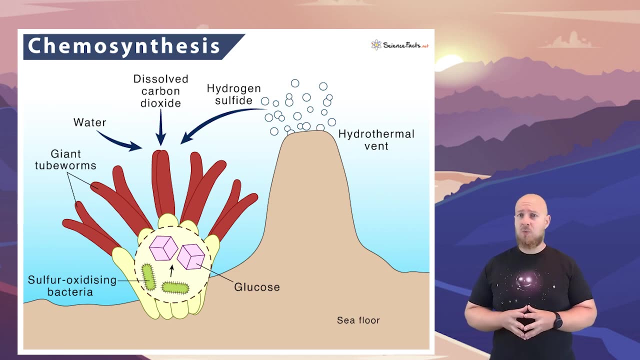 however, energy can still be produced even at the ocean floor, where there is no light, where producers instead undergo chemosynthesis. chemosynthesis is a way to make a glucose, but instead of it being powered by the light energy from the sun, it is being powered by 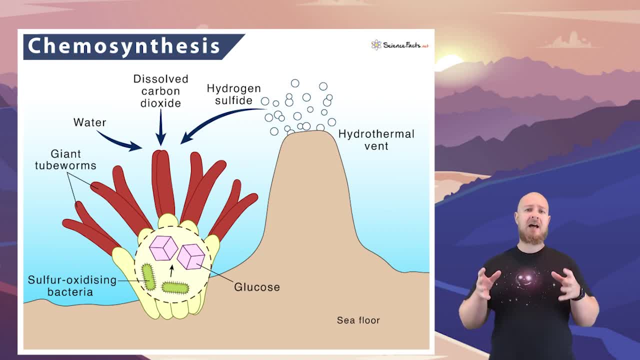 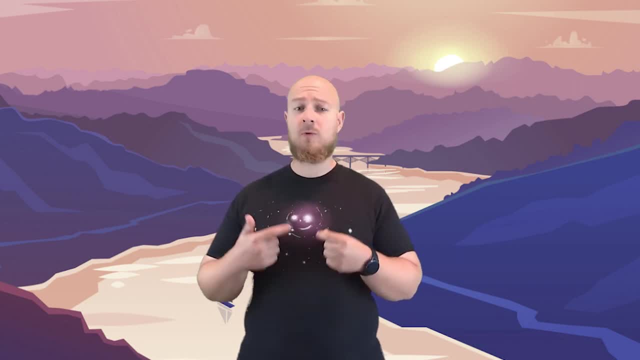 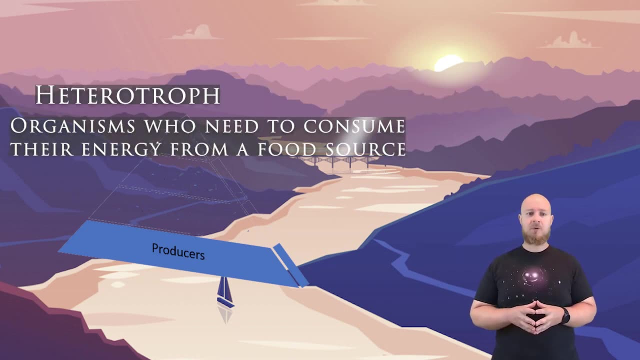 heat and chemical energy from hydrothermal vents and hydrogen sulfide. now that we've got energy available to the ecosystem, we can look at how that energy moves through it. producers are eaten by heterotrophs, or organisms who are unable to produce their own food, so they must eat in order to obtain energy. the first step of heterotrophs are the primary consumers, and these are organisms that are usually herbivores, meaning they almost exclusively eat plants, or omnivores that really eat anything above that. are secondary consumers: these are organisms that are usually omnivores or carnivores, meaning they eat meat or, better yet, secondary consumers. 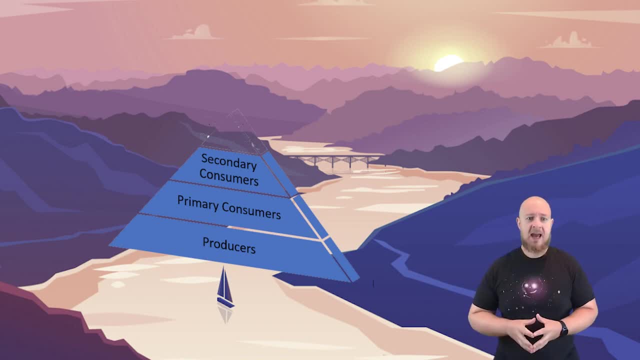 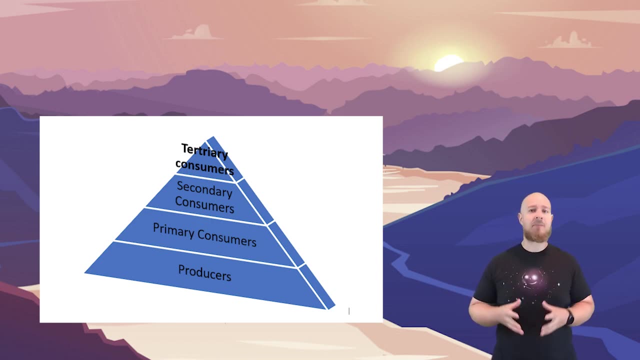 are things that eat. primary consumers at the top of this pyramid are the tertiary consumers, and these organisms are most commonly carnivores and top predators in an ecosystem. tertiary consumers consume secondary consumers. this model is called a trophic pyramid and each step is called a trophic level, as you go. 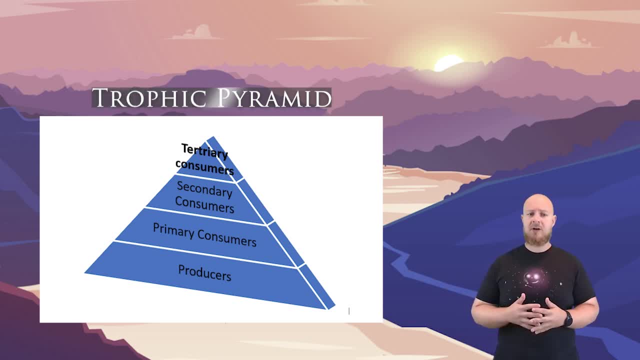 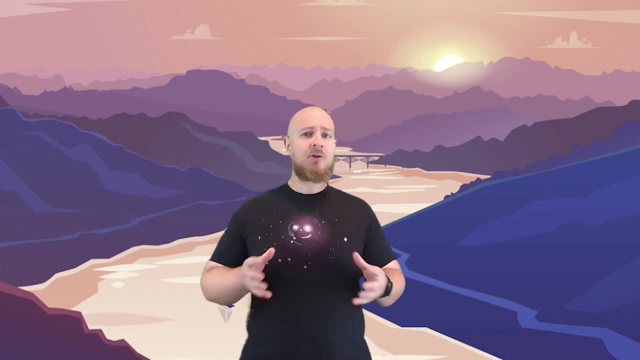 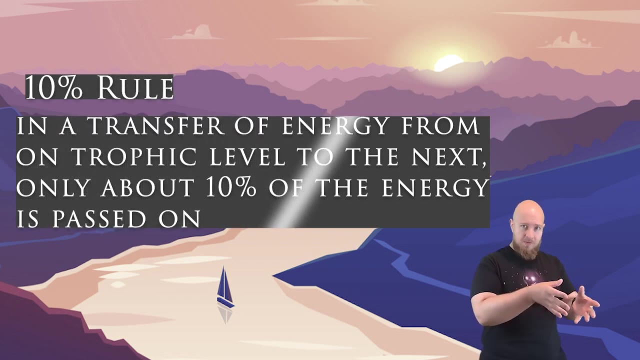 up in the pyramid. the subsequent steps acquire their energy from the trophic level below. this transfer of energy, however, is not very efficient. energy flow between trophic levels is described by the 10 percent rule, which approximates that in the transfer of energy from one trophic level to the next, only about 10 percent of the energy is passed on. so let's just say that in an ecological community all the producers contain one million calories worth of energy. this implies that the total caloric value of the primary consumers would be about a hundred thousand and the entire group of secondary consumers would contain ten thousand, and that means the entire set of tertiary consumers would contain only one thousand calories. 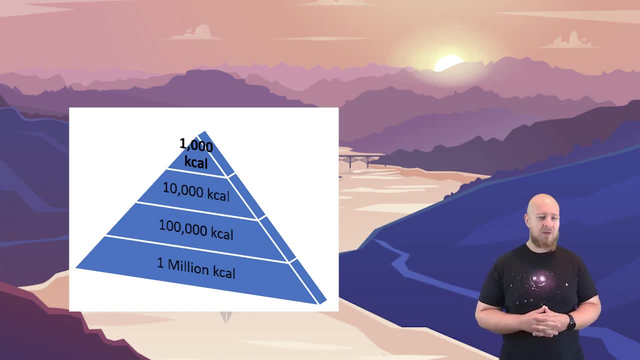 so this is a very important example of how the energy flows between these trophic levels. so what does all this energy go in between these trophic levels? well, a lot of it is lost as heat. remember the second law of thermodynamics that says energy conversions are not going to be. 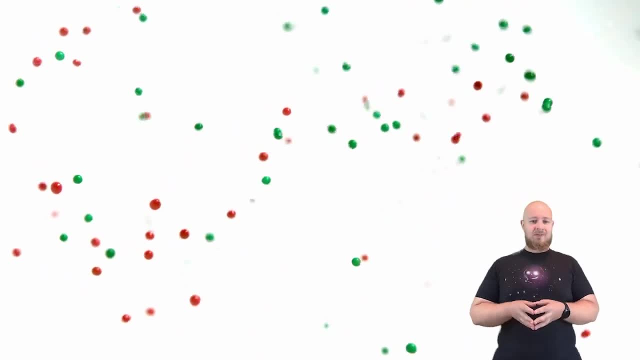 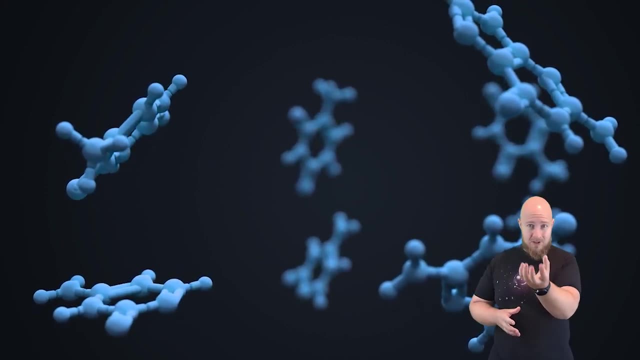 particularly efficient. the universe tends towards disorder. heat is a less ordered form of energy, as it really is just a measure of how fast particles are moving. the energy stored in your body, chemical energy, is very ordered, as chemical bonds generally don't move around as much so when 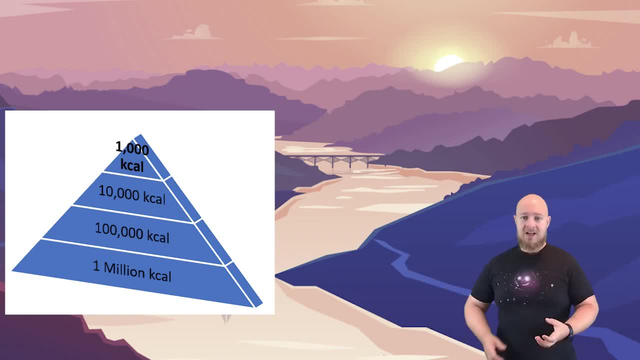 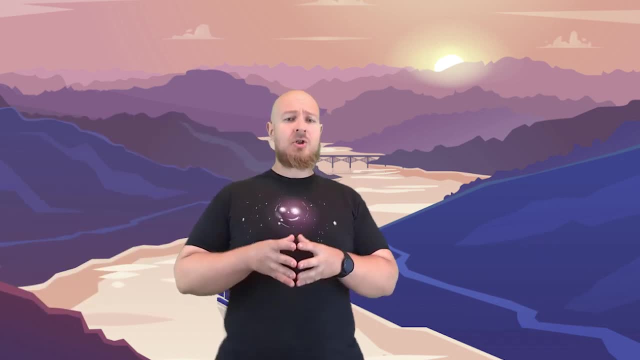 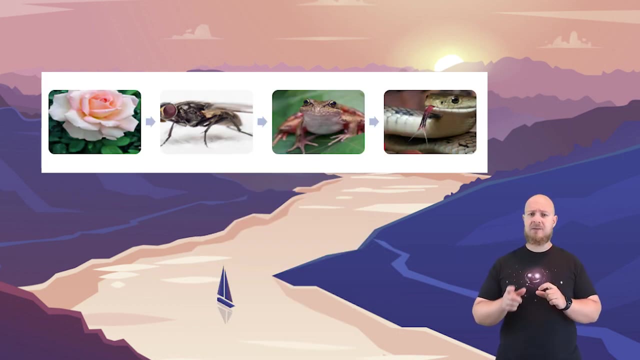 energy transfer occurs. it is so inefficient that about 90 percent of all that energy is lost as heat. a trophic pyramid can only tell us so much about the transfer of energy in an ecosystem. a food chain is a way to model how different organisms obtain their energy.